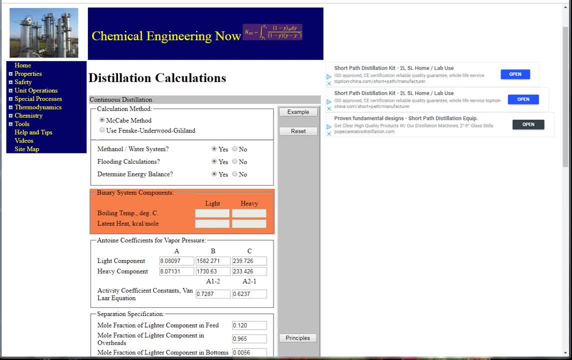 There are several distillation calculators at chemicalengineeringnowcom, such as Batch, Batch Column and Continuous. Today we will explore an example utilizing the Continuous Binary Distillation Calculator and McCabe method To set this up. we will create a material balance sheet with a system diagram and given data. 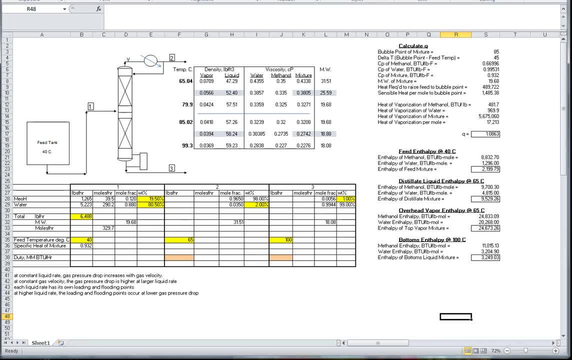 In this example, Distillation Column is to separate 6488 pounds per hour of feed mixture from a tank at 40 degrees centigrade and consisting of 19.5% methanol and the balance water. We wish to obtain 98% methanol on the top and 1% methanol on the bottom by weight. 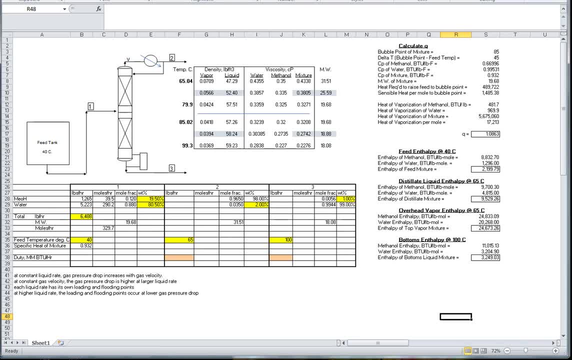 Converting the feed to mole fraction shows the feed consisting of 0.120 mole fraction of methanol and 0.88 mole fraction of water. Similarly, converting the column top and bottom streams to mole fraction shows that the top consists of 0.965 mole fraction of methanol. 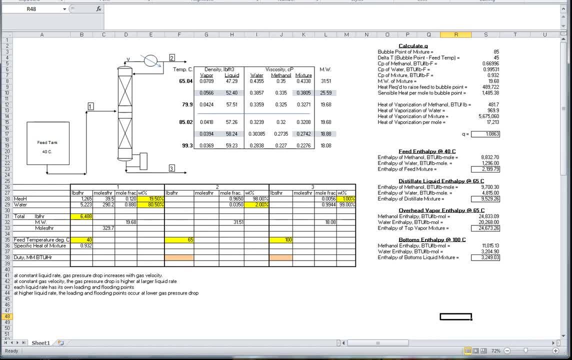 0.035 mole fraction of water and 0.880 mole fraction of water. In this example, Distillation Column is to separate 6488 pounds per hour of feed mixture from a tank at 40 degrees centigrade and consisting of 19.5的 water. 0.0056 of methanol. 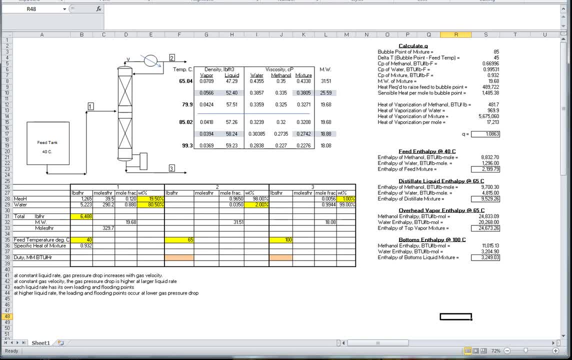 and 0.9944 of water. We could solve the simultaneous equations in order to complete the flow rates on the material balance, but the calculator will do that for us. We may have an existing column of known diameter or may try to determine the size of a new column. 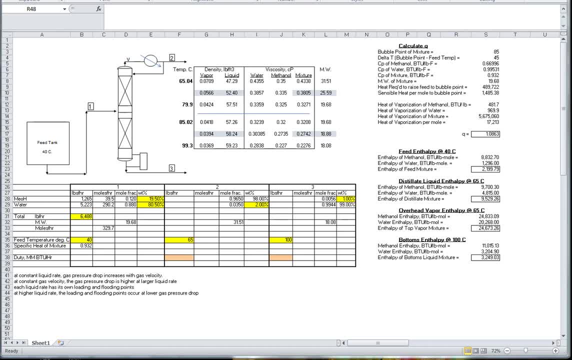 We will start by taking a column diameter of 3 feet in the rectification section and 3 feet in the stripping section, then explore smaller diameters. Each section is equipped packing that equates to a random packing factor of 25.. The packing factor is determined empirically. 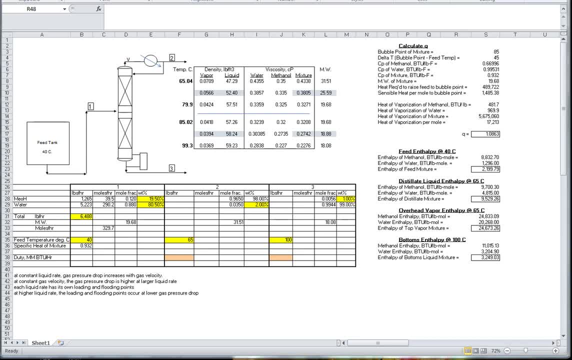 for each type of packing. Packing factors can be found in literature or obtained from packing manufacturers. for each type and size, The initial reflux ratio will be 1.5, but we will also investigate lower rates. So our procedure will be to calculate the number of separation stages. 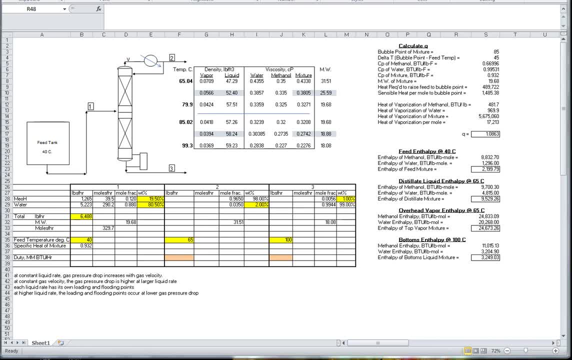 then calculate the flooding with the given column diameter and see the effects and change in the diameter, and then calculate the re-boiler and condenser duties for the given conditions. To determine the Q first. to determine the Q value in order to calculate the separation stages. 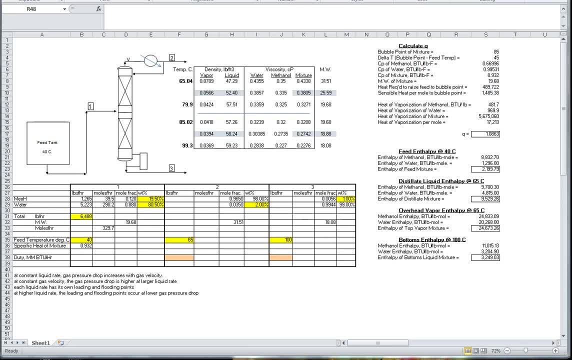 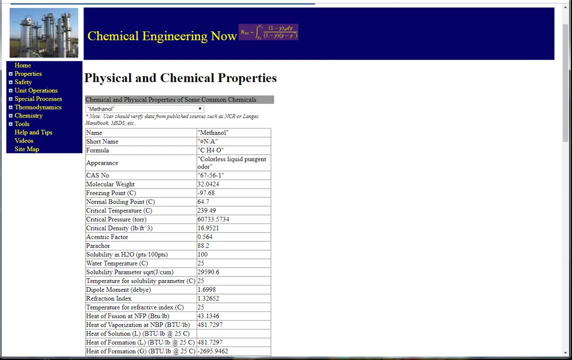 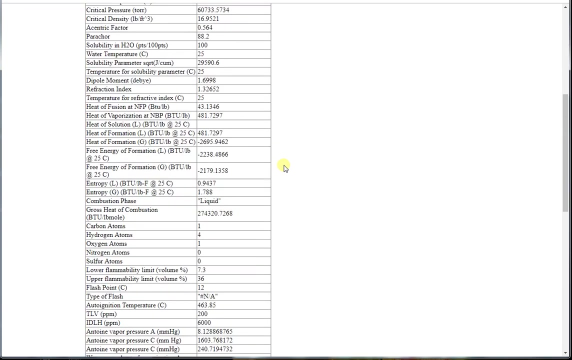 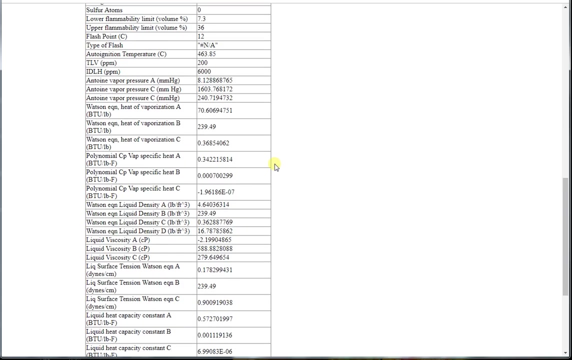 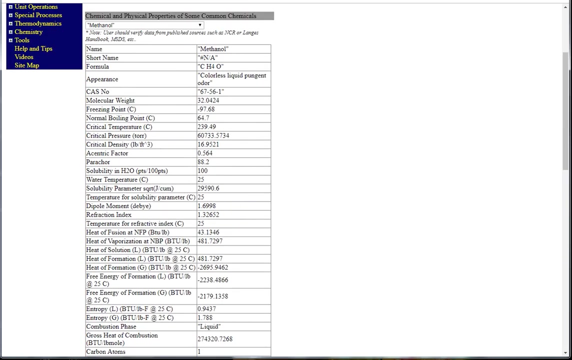 we must determine the bubble point temperature To get to the. so if we go to the physical and chemical properties pages chemicalengineeringcom, we can find the physical properties and polynomial equations for physical and thermo data. We can use this information in determining bubble point and. 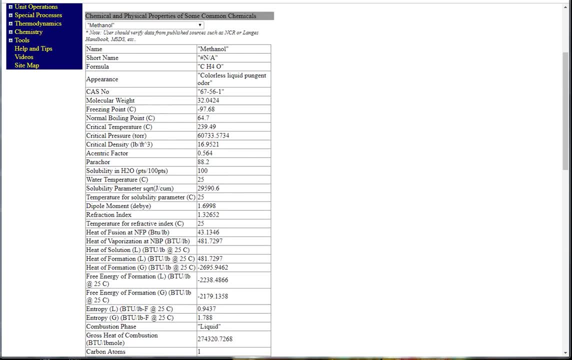 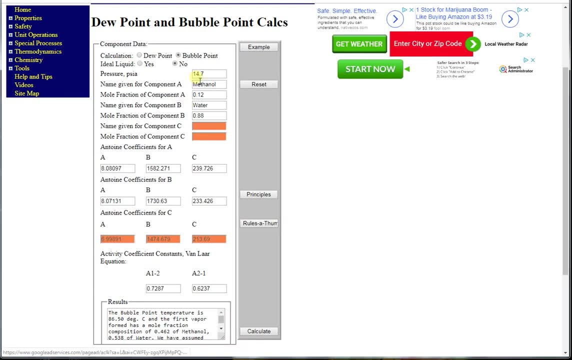 solving the other, solving for the other data necessary in our calculation. If we take this information, we go over to the bubble point calculator and we input our feed conditions, the Antone coefficients, the activity coefficients, Since methanol and water is a non-ideal liquid mixture. 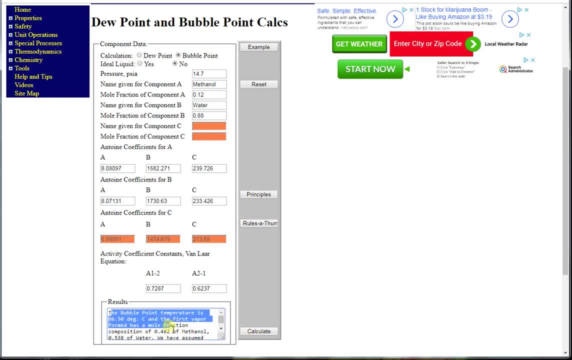 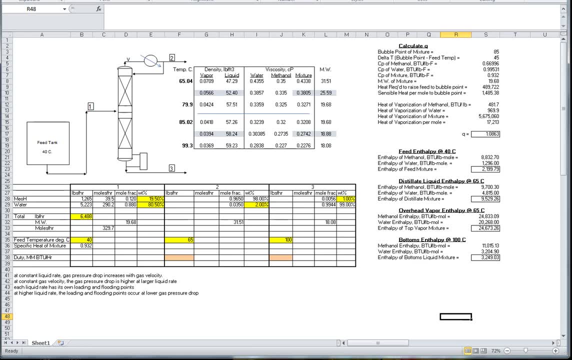 we calculate that the we can calculate the bubble point temperature. Now, if we take this bubble point temperature over to our calculator, we can calculate that the delta, the delta temperature, is 1.6 and 2.7.. the delta temperature of the feed. Then, using the, 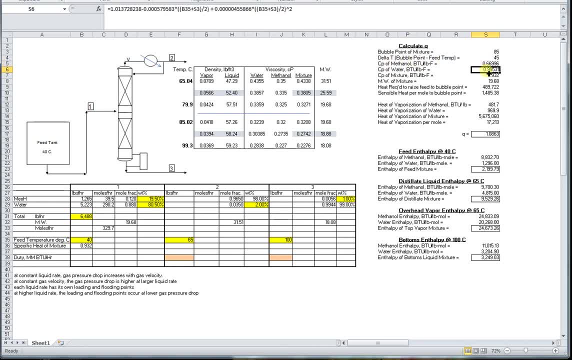 polynomial equations we can calculate the specific heat and the amount of sensible heat necessary to raise a mole from the feed temperature to the bubble point temperature. Similarly, we can use our equations to calculate the heat of vaporization of a mole feed, and with that we can calculate the Q value. 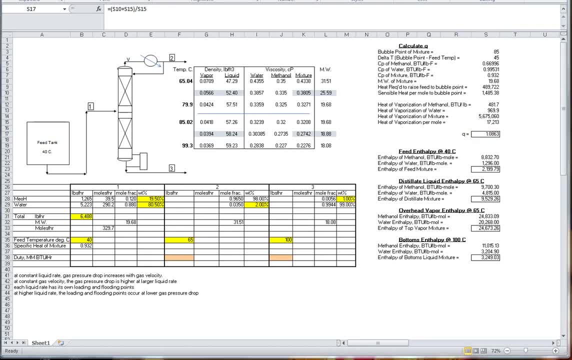 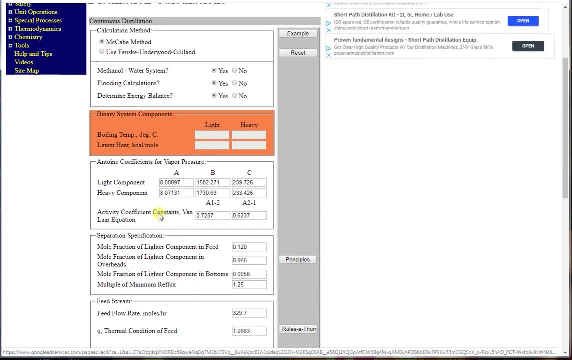 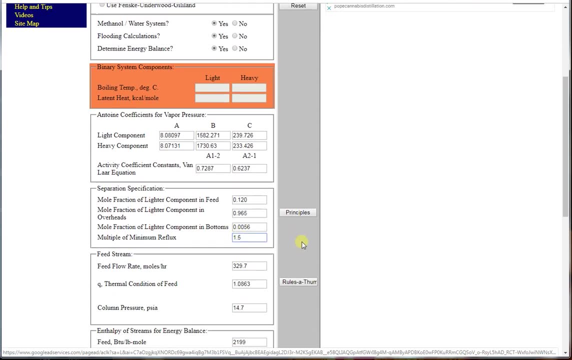 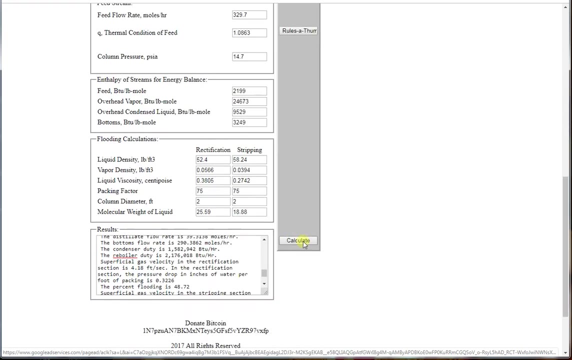 Now, with this Q value, we can go back to our calculator and we can input again the anitone coefficients, the activity coefficients, our feed concentrations, our reflux ratio of 1.5, our feed rates, our Q value, and we can determine. 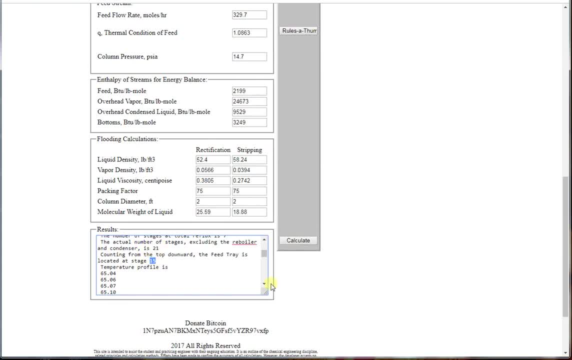 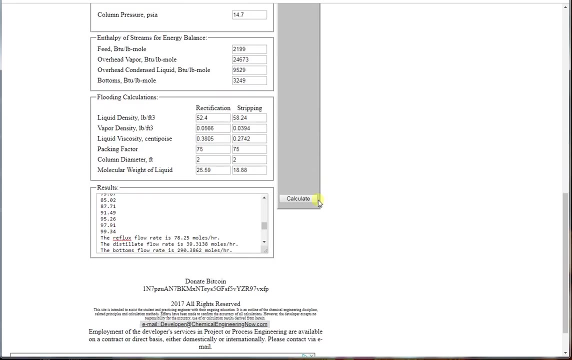 the number of stages, the feed stage, and we can see the profile across the column. If we want to reduce and see the effect of reflux rate, we can do that, and by doing so we see that the number of stages goes up to 25.. So it's just a good design. 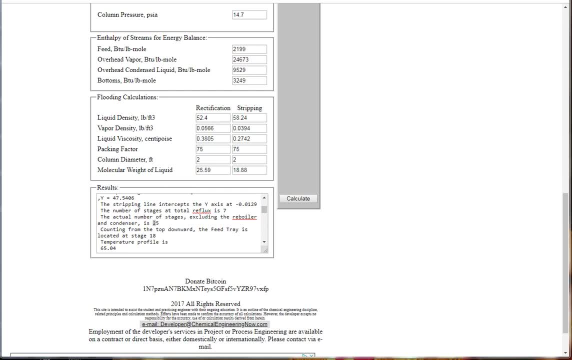 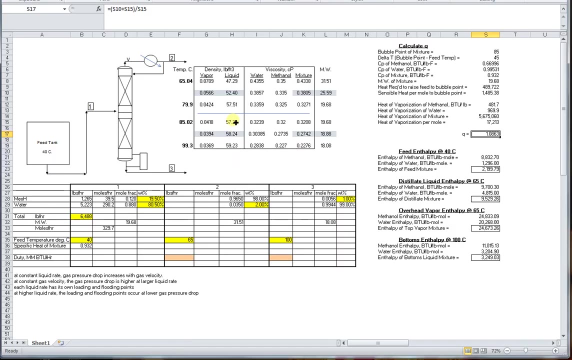 We need to check column flooding and then consider the trade-off, So among column height, column diameter and exchanger sizes duties. So next calculate the flooding with this column diameter and see if another diameter would be better. The table in the middle of this spreadsheet shows the temperature profile across the column. 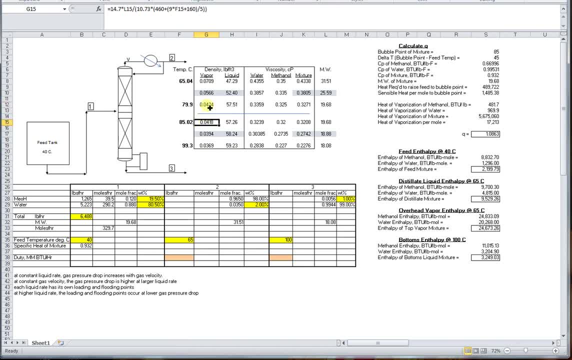 The top, the bottom, above and below the feed. We've also calculated the densities of the vapor, the liquid and the heat, The vapor, the liquid, the viscosity of the mixture at each stage. Then we've taken the linear average between these stages. 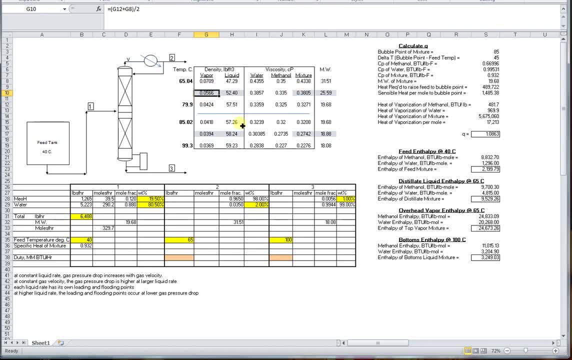 to calculate an average of the middle of the bed And we're going to use these values in our calculator. But it is advised that the viewer check the top and the bottom of each section for flooding. So if we put this data into our calculator, 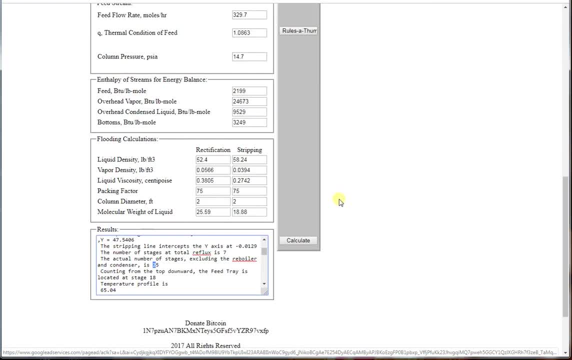 We run the calculations again. We have this data now here in the flooding calculator section. We find that the well, we have three feet. We find that the flooding in the rectification section is 21.. And in the stripping section is 22.. 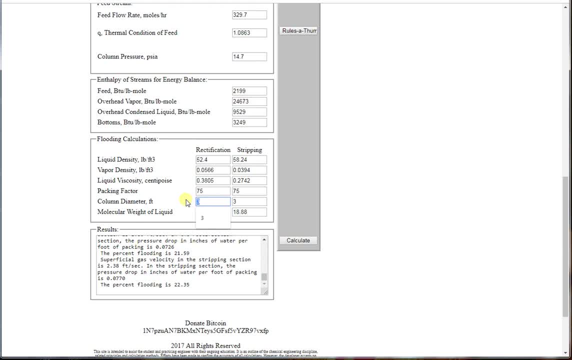 Rather low values. If we want to see the effect of a two foot diameter column, We see, now that our flooding has gone up, 48 and 50. Maybe more, maybe better values, maybe a better design. Next, we want to calculate the reboiler duty.